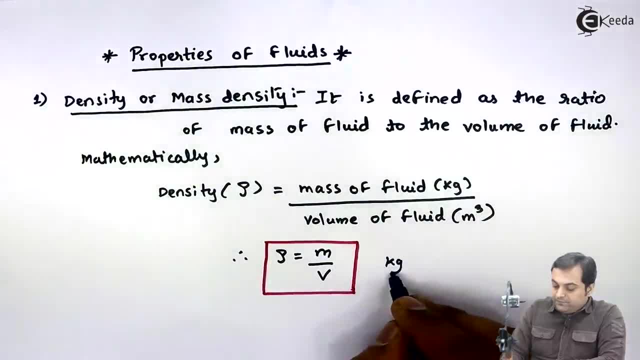 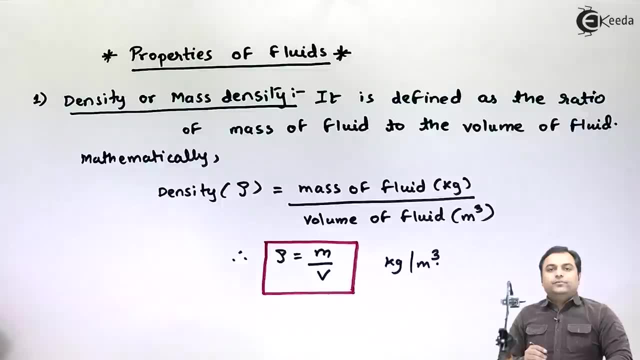 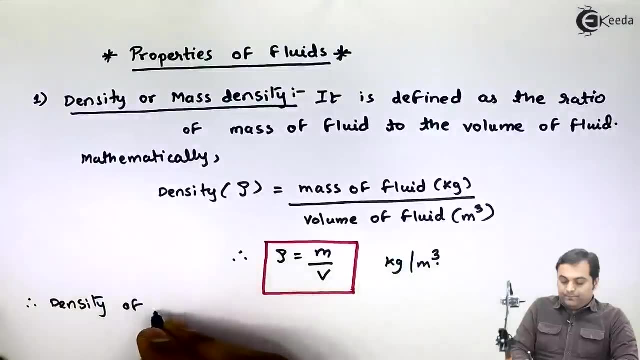 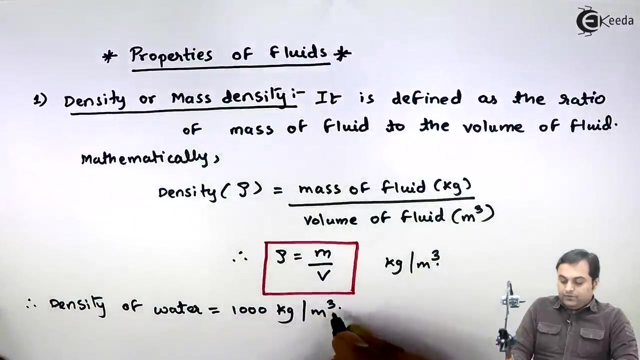 And the unit we have. it is kg per meter cube. Next, density for standard liquid, and standard liquid will be water for us. So I will write down there: for density of water It is equal to 1000 kg per meter cube. This is the standard, or we can say the reference liquid. 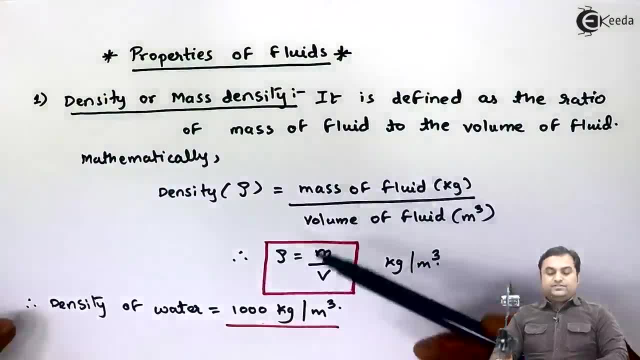 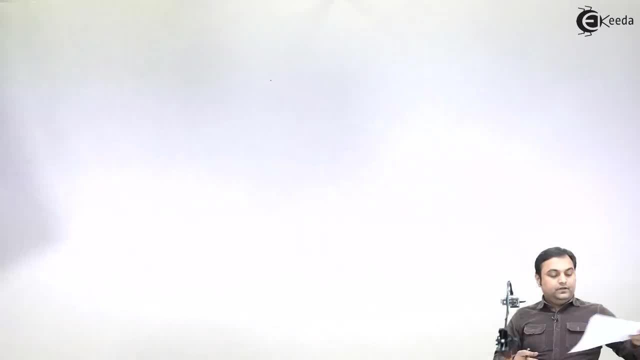 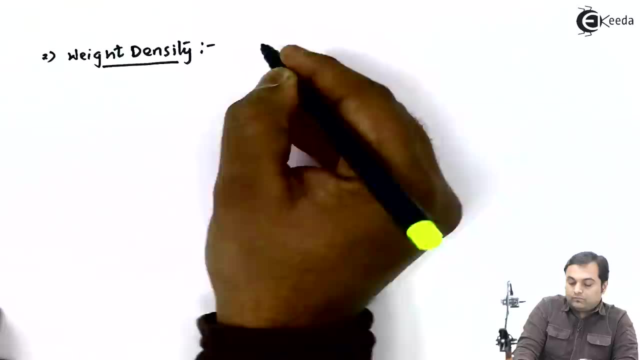 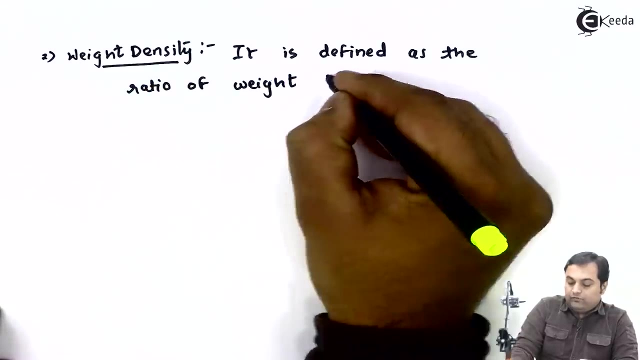 So this was regarding the mass density, that is, it is defined as the ratio of mass of fluid to the volume of fluid. The next property that is called as weight density. It is defined as the ratio of weight of fluid to the volume of fluid. 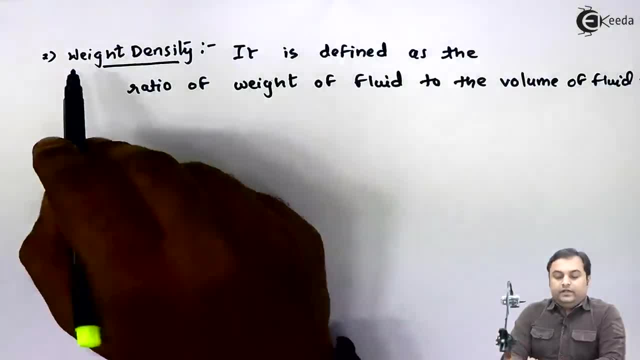 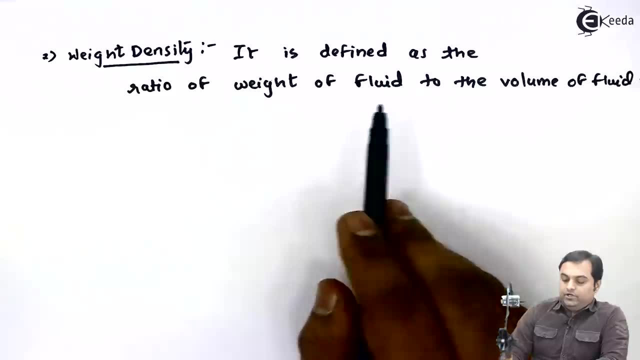 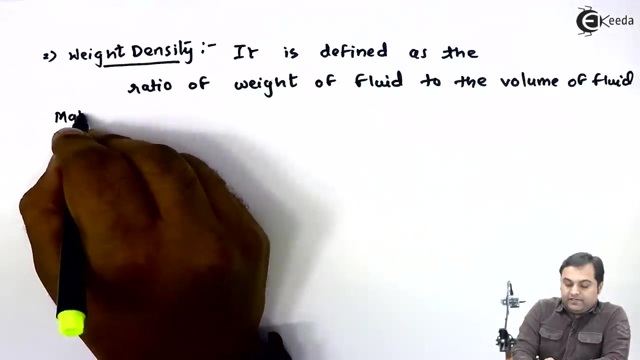 So here is the definition of weight density. In mass density it was mass upon volume, That is, it was the ratio of mass of fluid to the volume of fluid. Here we have the ratio of weight of fluid to the volume of fluid, And mathematically it can be written as: 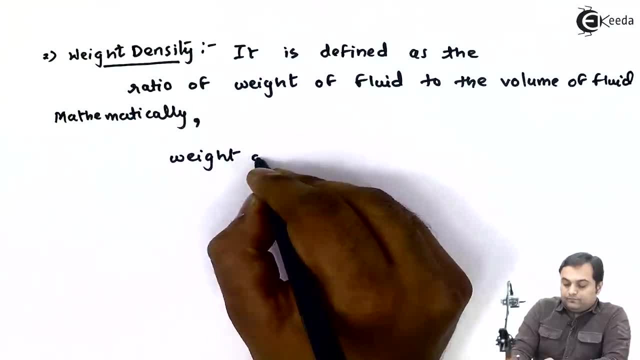 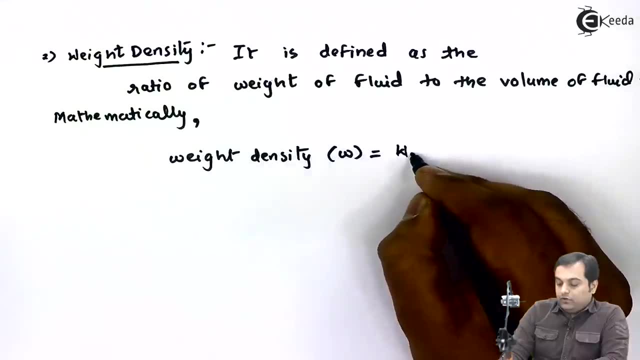 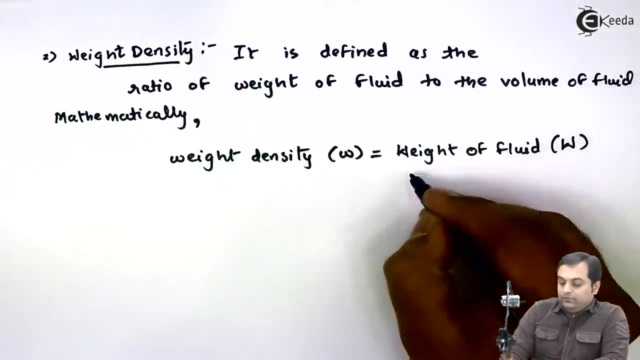 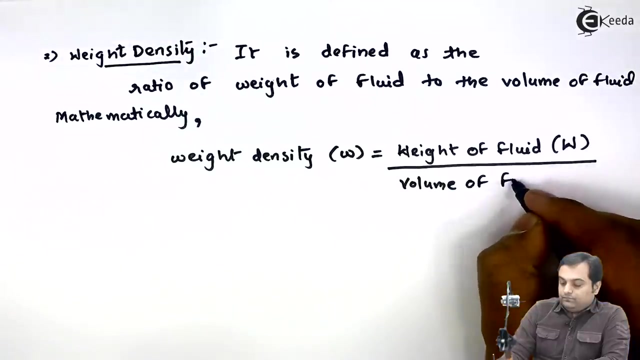 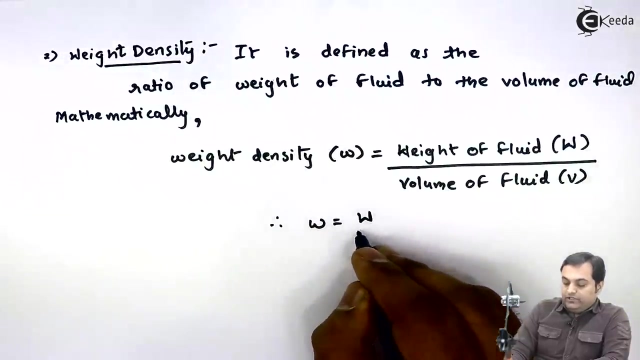 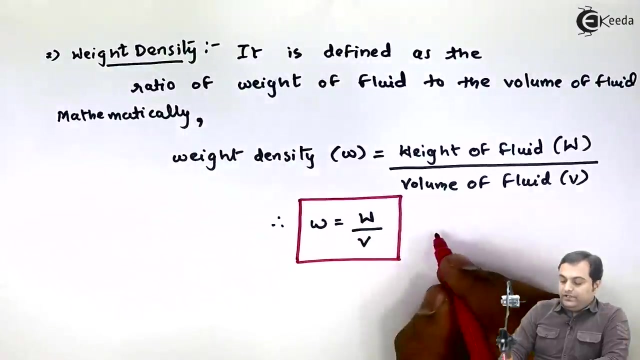 weight density. it is denoted by small w. that is equal to weight of fluid capital, W divided by the volume of fluid, Which is denoted by W. So therefore, weight density becomes weight upon volume. Unit will be weight in terms of Newton, volume is in terms of meter cube. 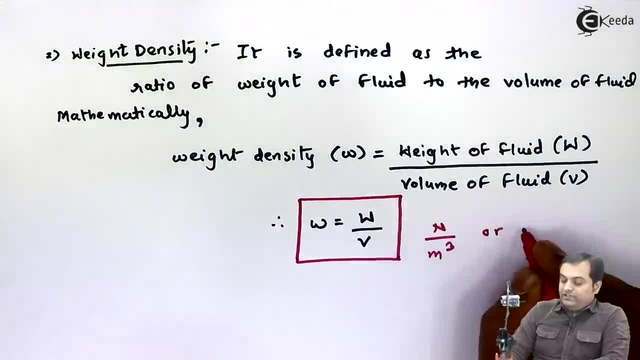 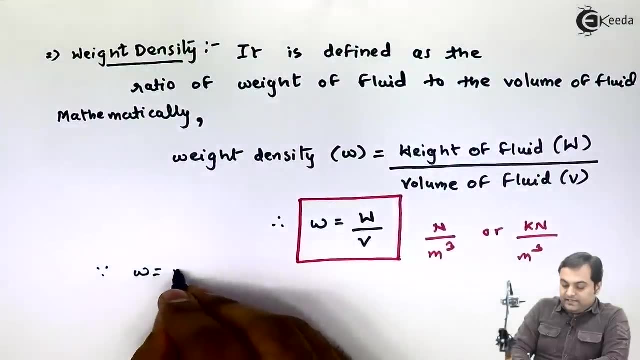 So Newton per meter cube, or if the weight is in terms of kilo Newton, So it is kilo Newton per meter cube. Next, we can even write down weight density, as, since W is equal to weight, can be written as M into G, that is, mass into acceleration due to gravity. 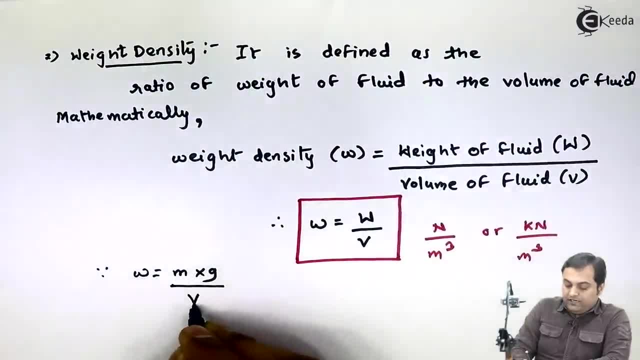 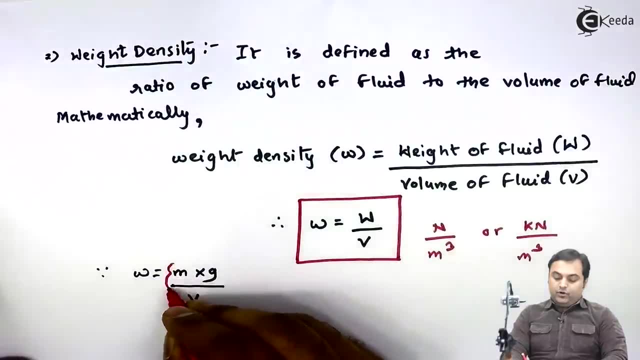 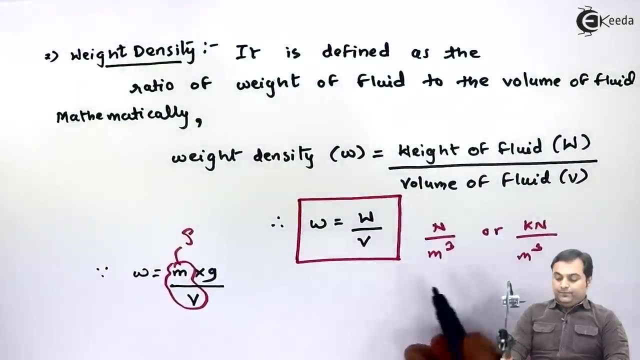 upon volume, Because we know that weight is equal to M into G. Now, as we see here, this term M upon V, that is, mass upon volume, is nothing but weight density rho. So therefore we have the relation, that weight density, or you can say that: 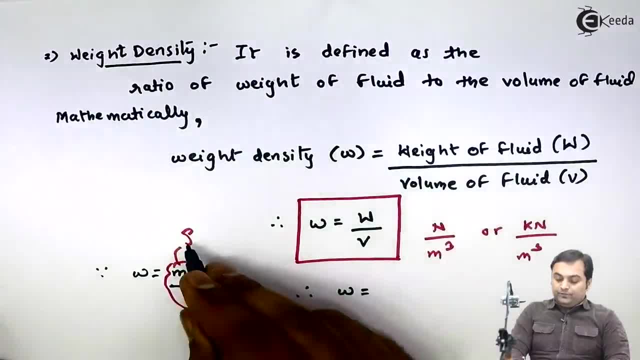 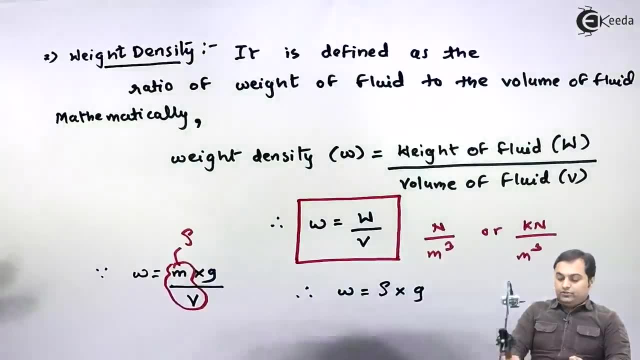 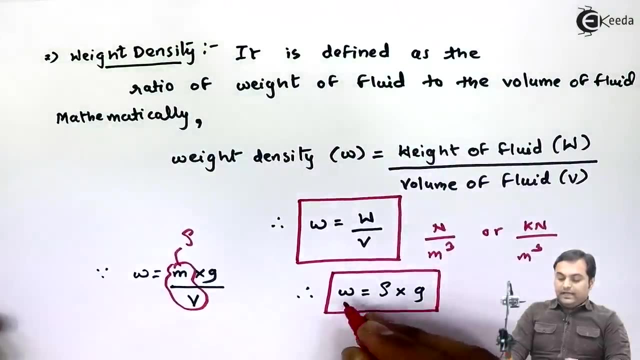 it is also called as specific weight. it is equal to rho into G, that is, mass density, into acceleration due to gravity. So here we have one more relation between weight density and mass density And this W, this weight density term. it is also called as specific weight. 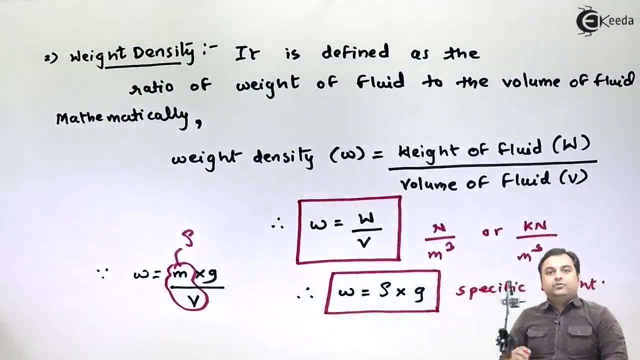 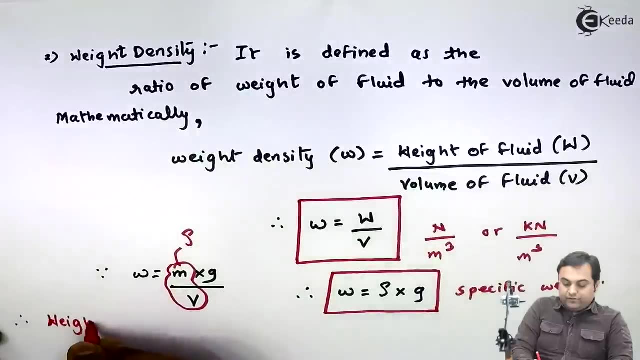 So if anywhere in the question they are mentioning that we have to calculate, or if they give the value of specific weight, specific weight is nothing but weight density of a fluid. Now here I can say that, therefore, weight density of water, because we are considering water as the 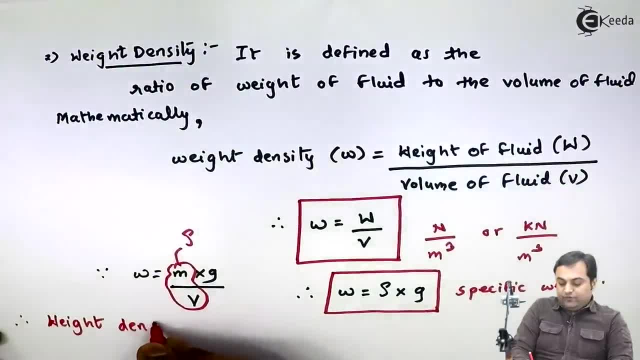 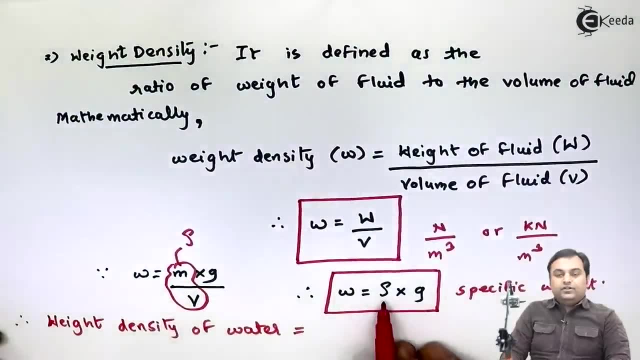 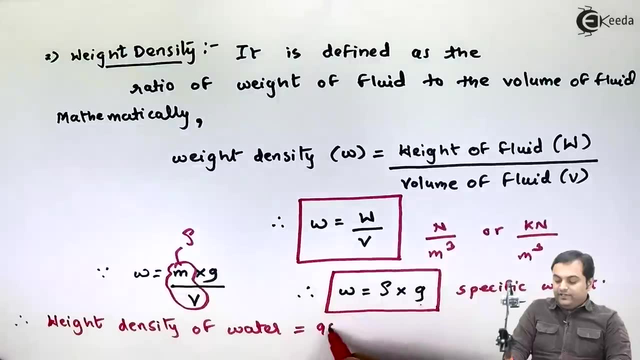 standard liquid. So weight density of water that is equal to, since rho value for water it is 1000. G is 9.81. so 1000 into 9.81 that gives me 9810 Newton. So this is the weight density of water. 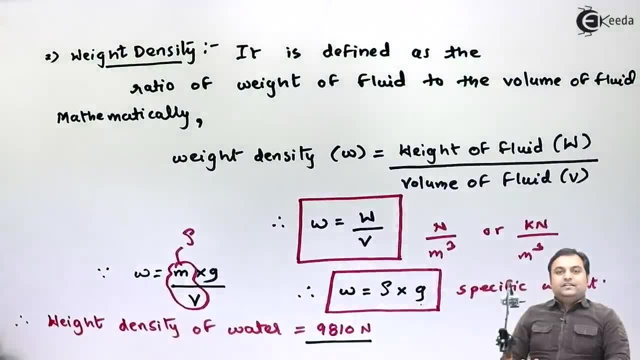 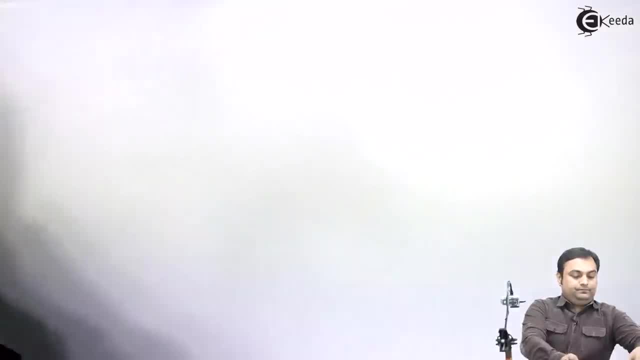 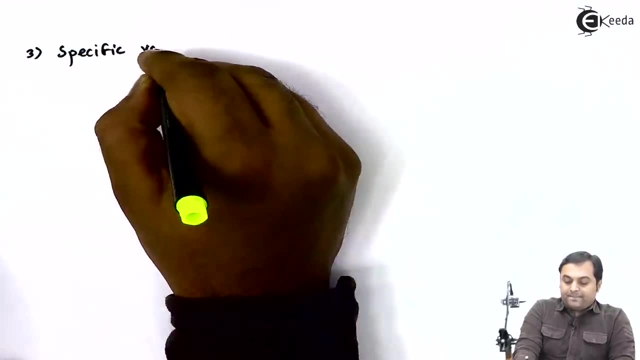 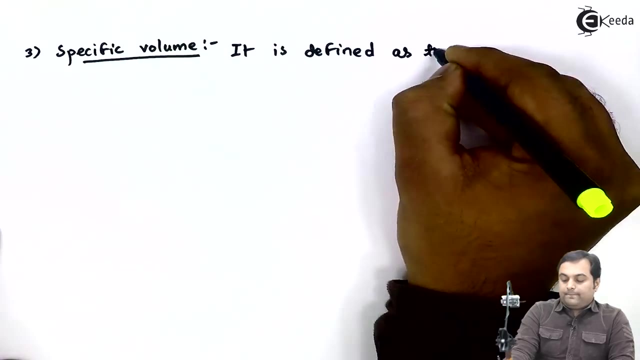 So, as we have seen the previous two definitions: mass density, it was mass upon volume. Weight density, it is weight upon volume. The next property: it is called as specific volume. Now, specific volume: it is defined as the ratio of of volume per unit mass. 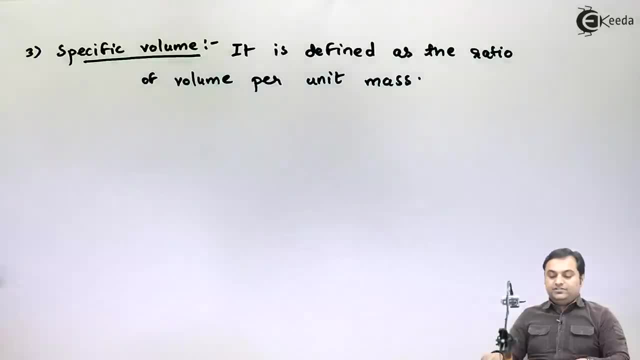 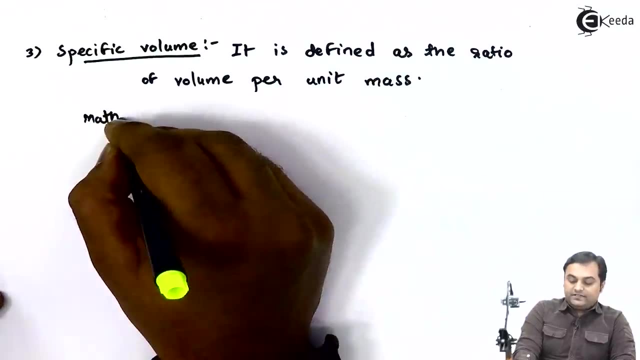 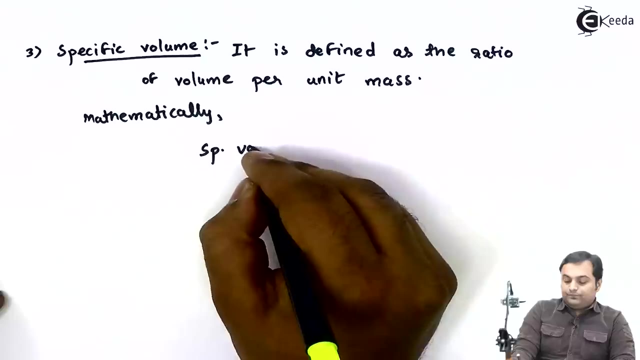 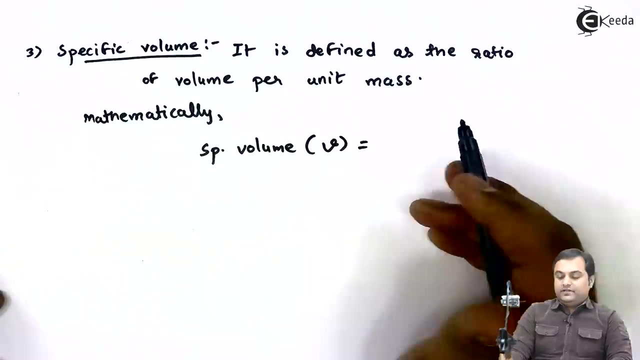 So we have another property, that is, specific volume, which is defined as the ratio of volume per unit mass, and hence mathematically it can be written as specific volume. it is denoted by a small letter. v is equal to the ratio of volume per unit mass. 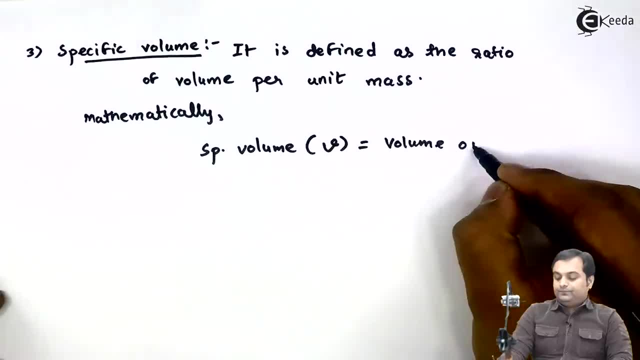 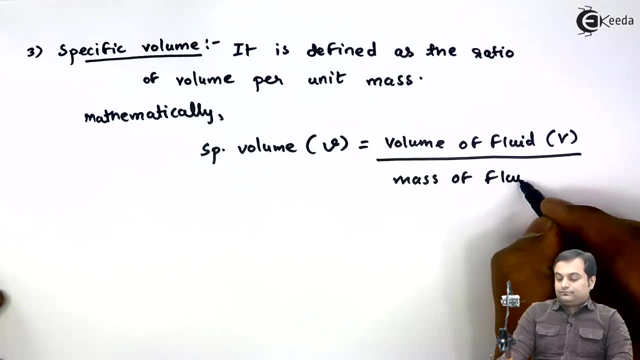 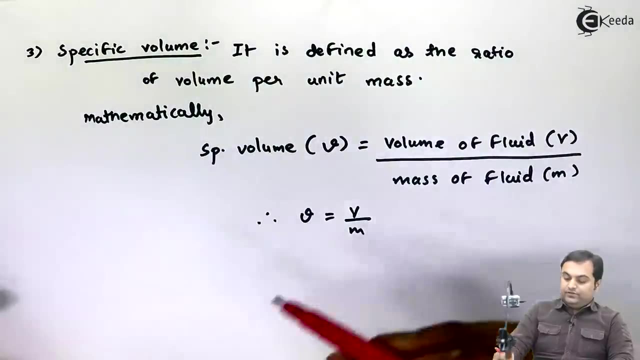 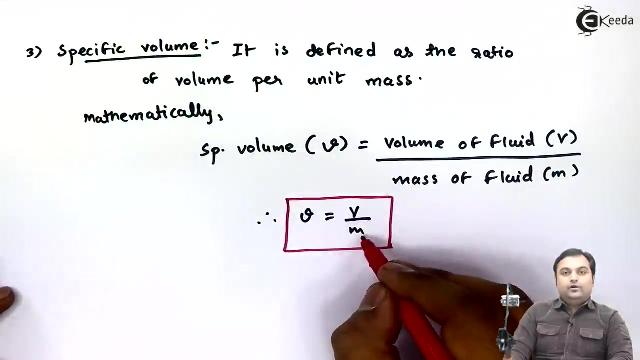 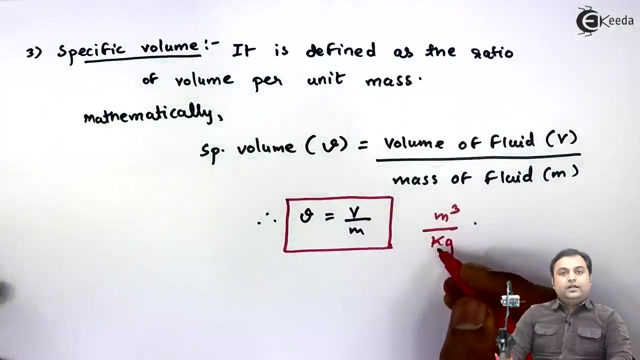 So it is volume of fluid upon mass of fluid. so therefore specific volume is volume upon mass and the unit will be, since we have volume upon mass, so it is meter cube per kg. that is the unit. If we see here, density was mass upon volume. 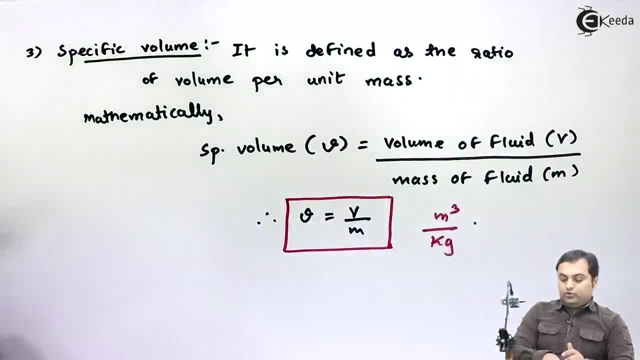 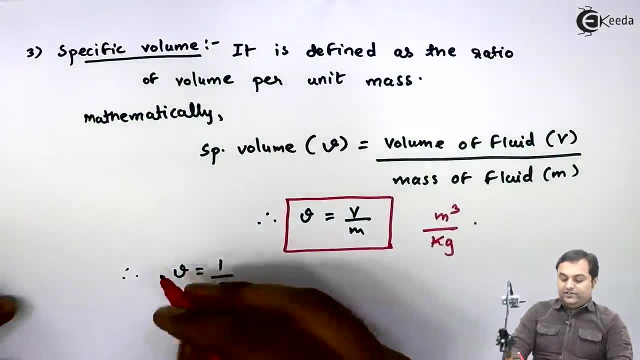 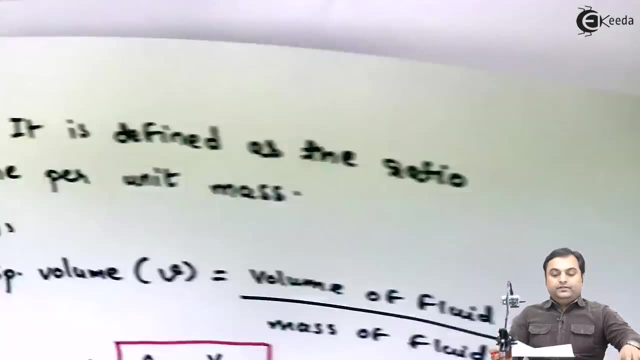 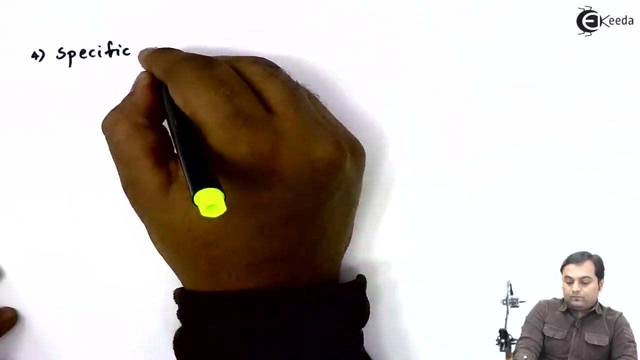 And specific volume is volume upon mass. So we can say that, therefore, specific volume is nothing but the reciprocal of mass density. One more relation we get here. So this is the specific volume. The next property that is called as specific gravity. Now, specific gravity. 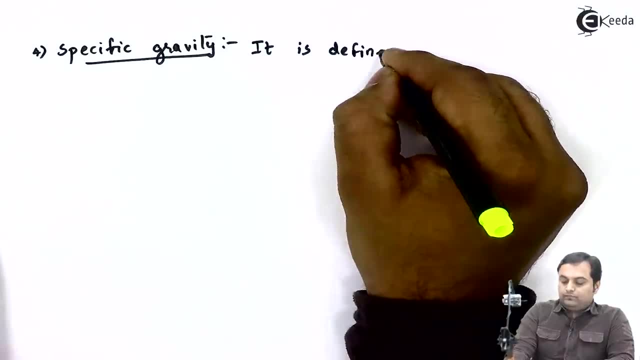 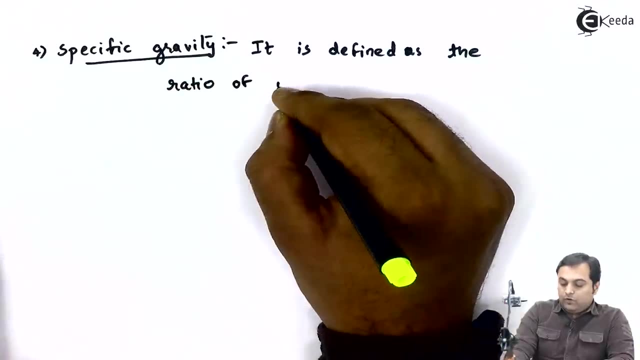 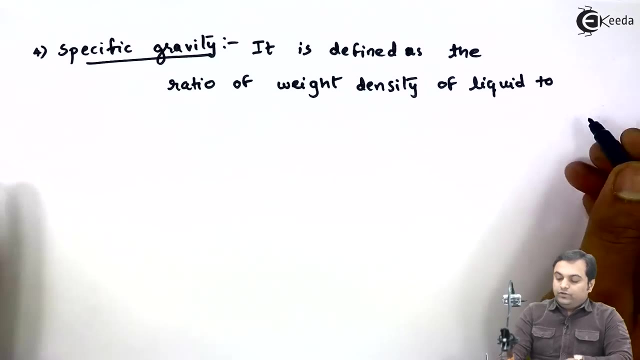 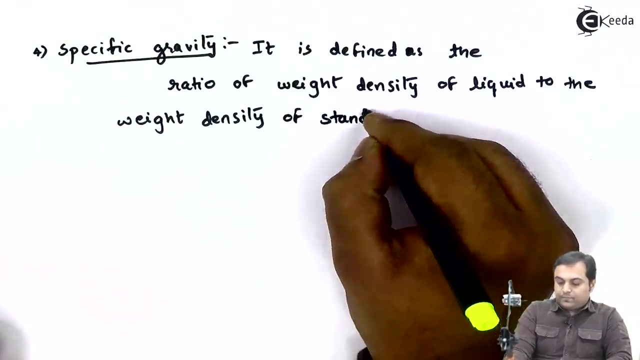 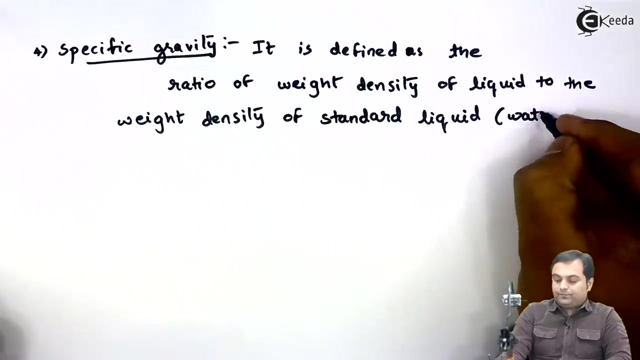 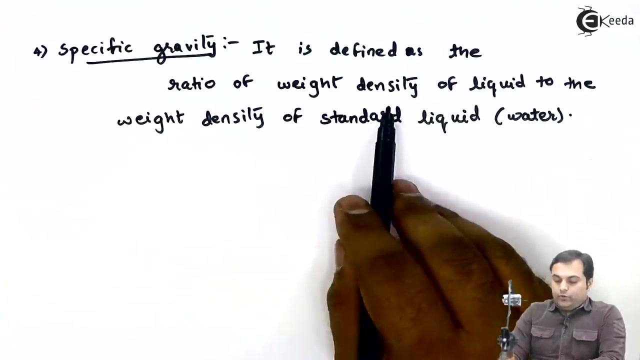 it is defined as the ratio of weight density of liquid to the weight density of standard liquid. And standard liquid we are taking it as water. So here is the definition. Specific gravity: it is defined as the ratio of weight density of liquid to the weight density of standard liquid. 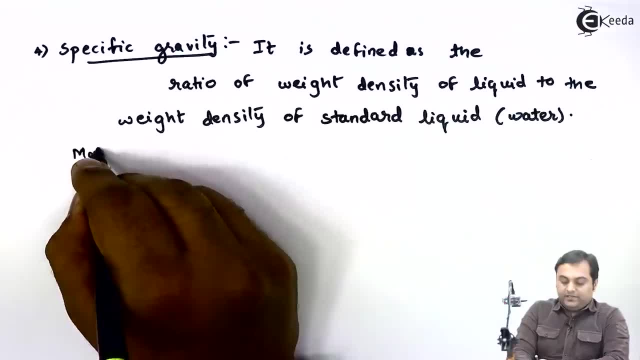 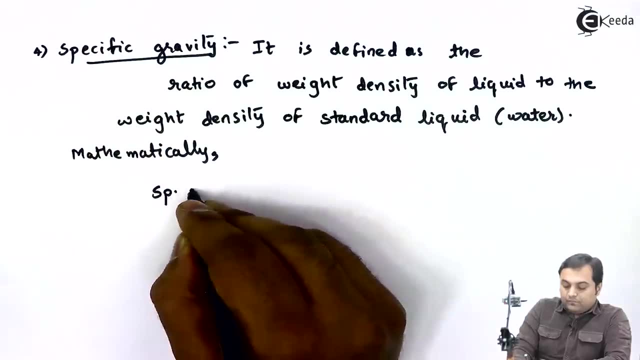 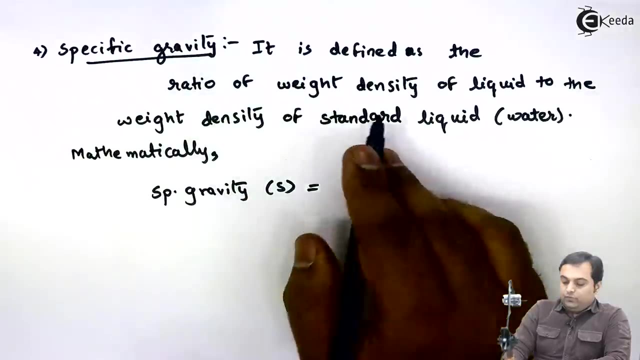 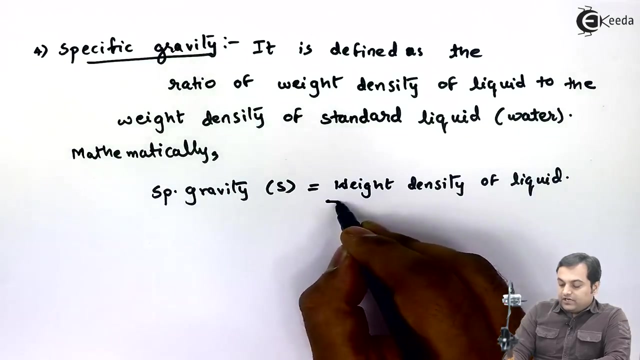 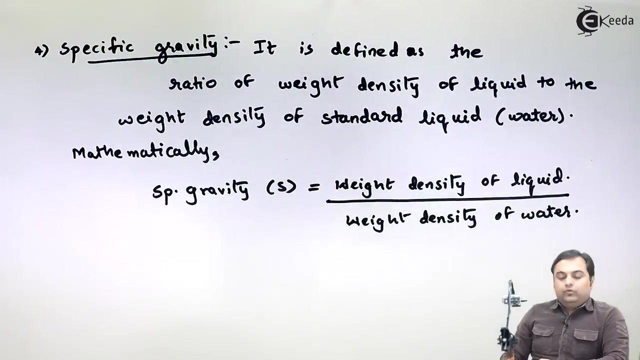 that is water, And mathematically this relation can be written as specific gravity. It is denoted by a small letter, s. It is equal to weight density of liquid, to the weight density of standard liquid. Here we are considering water. So if for any given liquid, 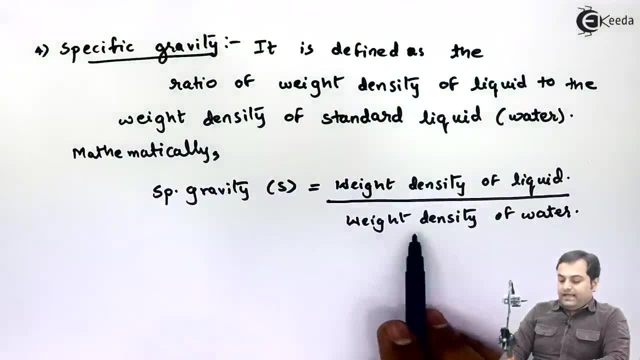 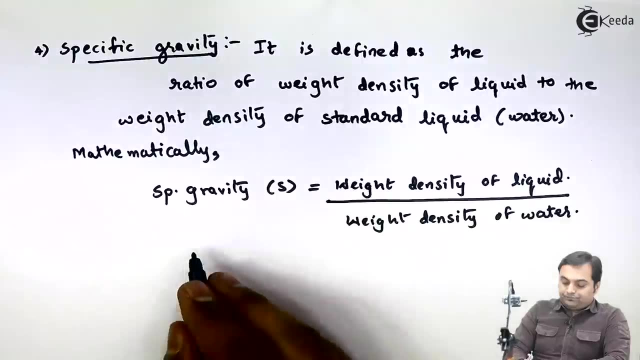 we know the value of specific gravity and we know the value of weight density of water, then we can get the value of weight density of that particular liquid. Now, this weight density- since here I have written weight density term- then specific gravity will also be equal to. 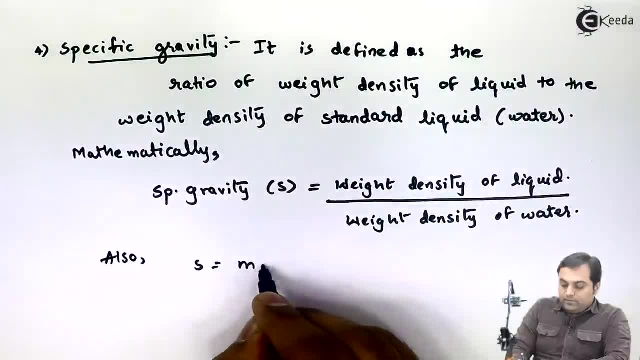 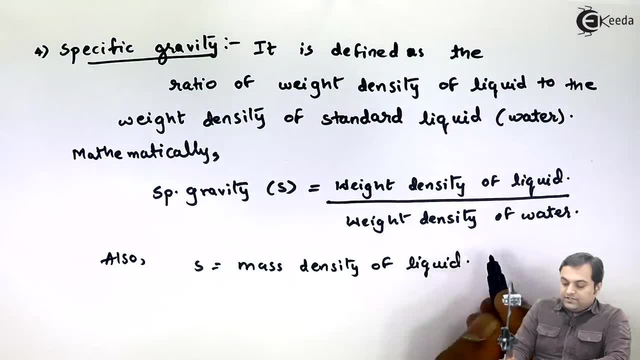 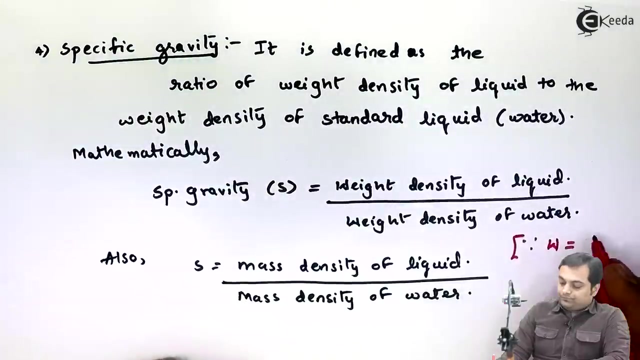 it is also: s is equal to mass density of liquid upon mass density of water. Why I have written this is that because, since weight is equal to mass, into acceleration due to gravity. therefore we know the relation. from that, we can say that the weight density which we have got previously 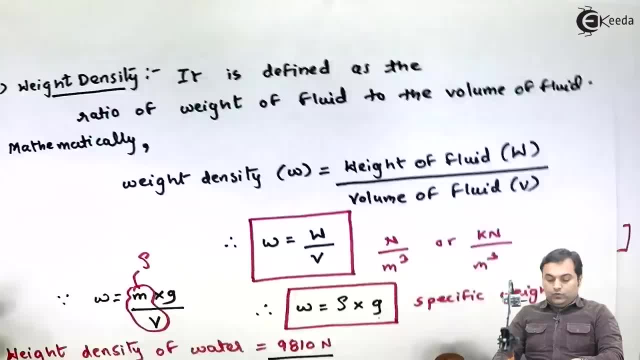 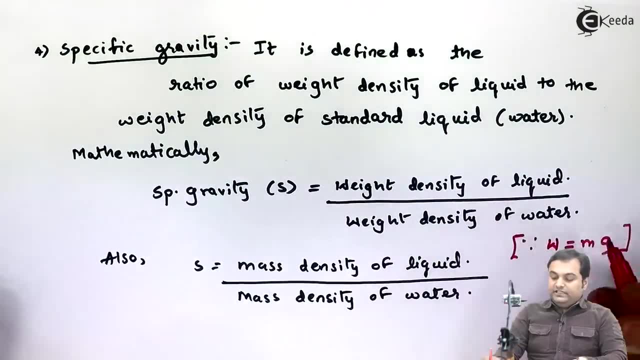 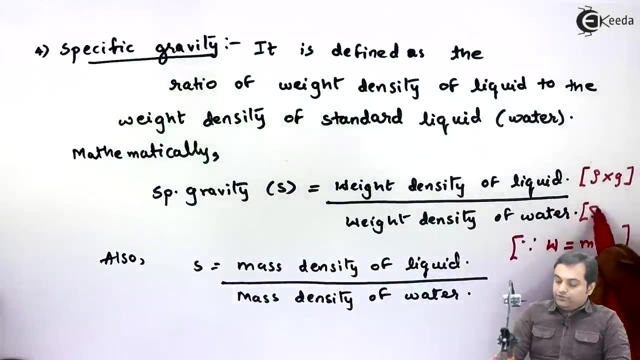 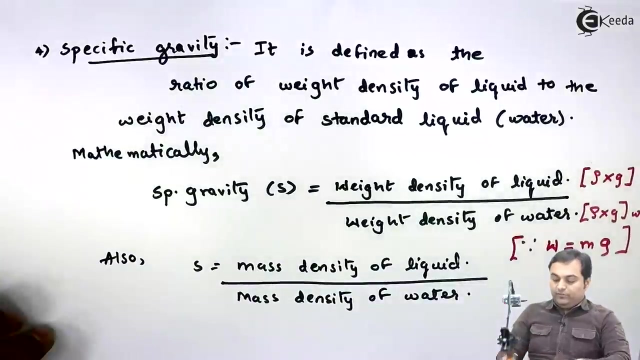 weight density is equal to rho into g. that is, if I write, instead of weight density of liquid, rho into g for liquid, upon rho into g for water, then g, g will get cancelled out, and here we have the formula of mass density of liquid, which is rho. 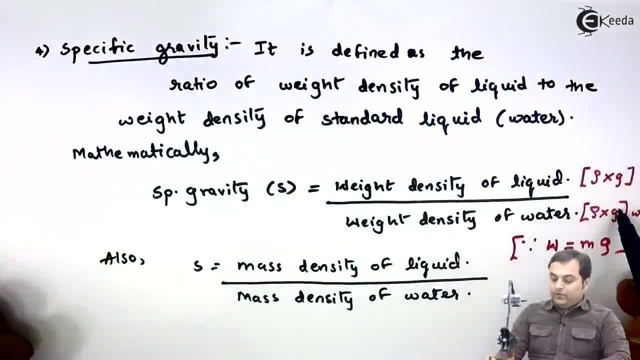 upon the density of water, so g gets cancelled out from both the sides. so in short, we can say that specific gravity can be written in both the form: in the form of mass density, in the form of weight density. specific gravity is weight density of a particular liquid. 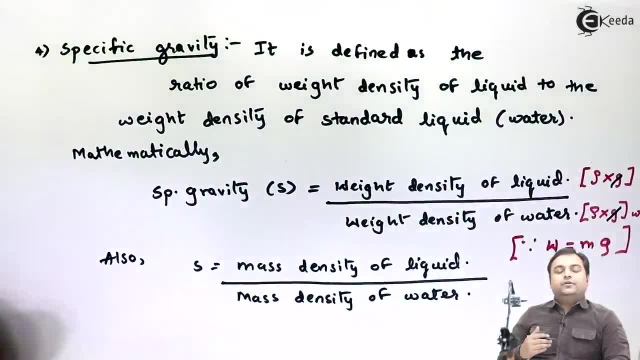 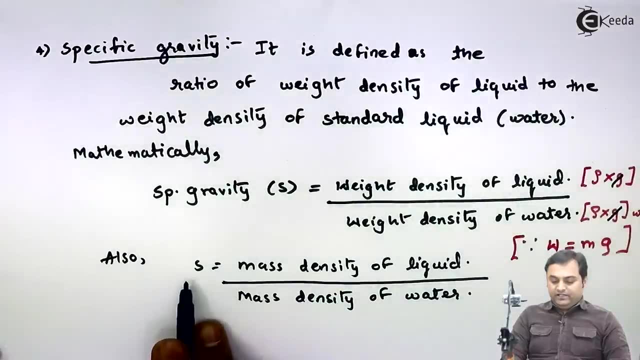 upon weight density of water, which is the standard liquid. specific gravity can also be written as mass density of a liquid divided by mass density of water. so I have written it here. suppose, for example, the mass density of a liquid. we know that specific gravity, specific gravity, is denoted by letter s. 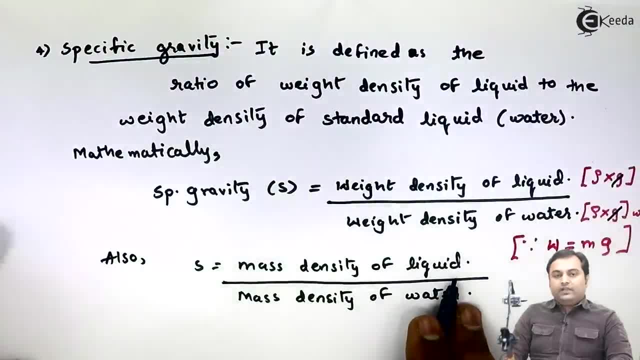 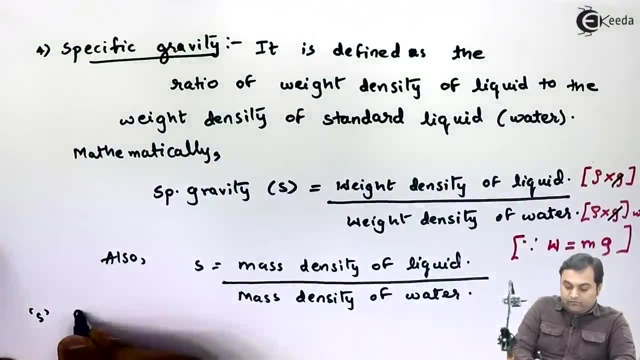 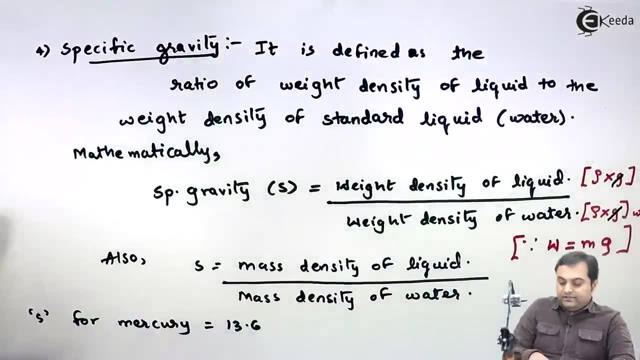 now mass density of liquid as mercury. if I am considering the liquid to be mercury, then I can say that s for mercury. it is equal to 13.6. that is, the specific gravity of mercury is 13.6. it means it is 13.6 times. 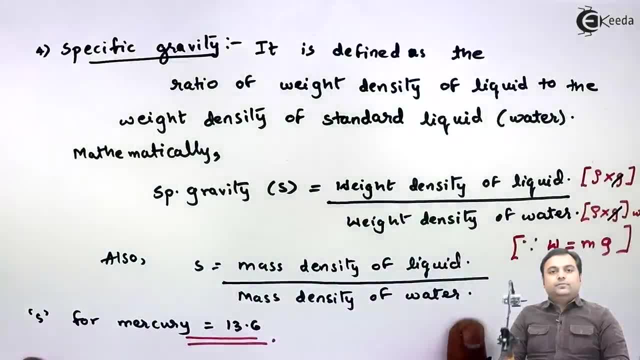 heavier than that of water, because the mass density of water will be 1000, but the mass density of liquid- if I am considering mercury, it will be 13600, so the specific gravity for mercury is 13.6. so once we know the relation between mass density,